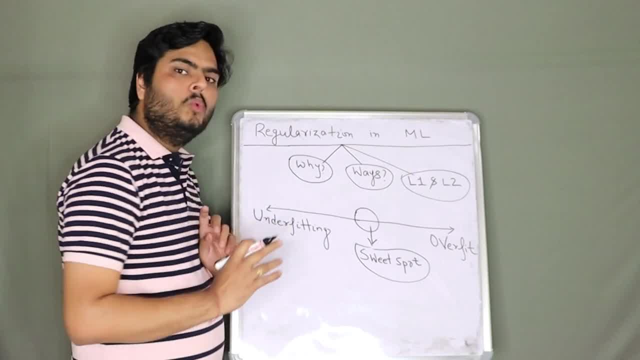 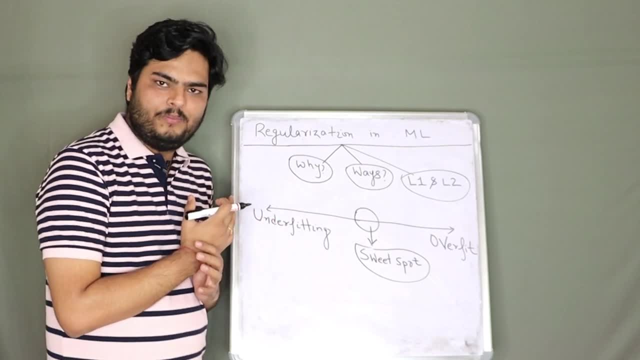 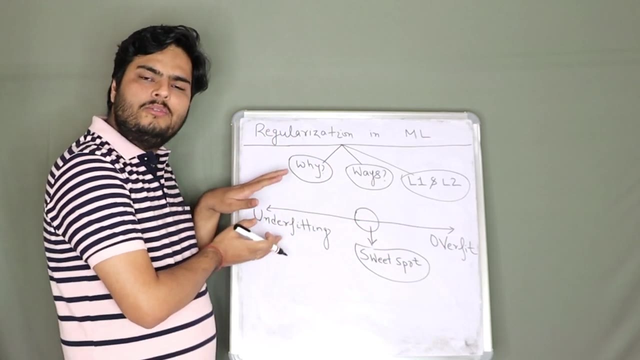 and due to other reasons as well, model over fits. What is the, what is the practical implication of model overfitting? model will kind of hug the data. it will remember the data and model is not flexible enough. here model is not learning enough and here model is not flexible enough. so what we have to find is: 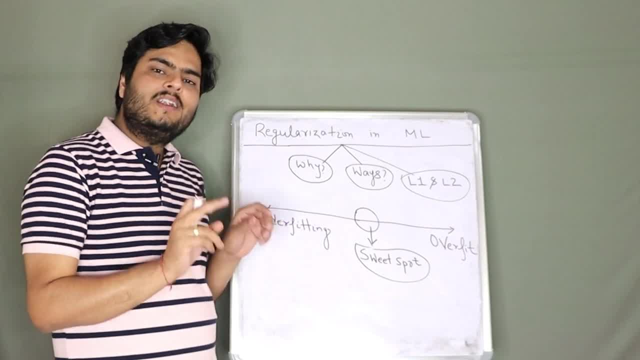 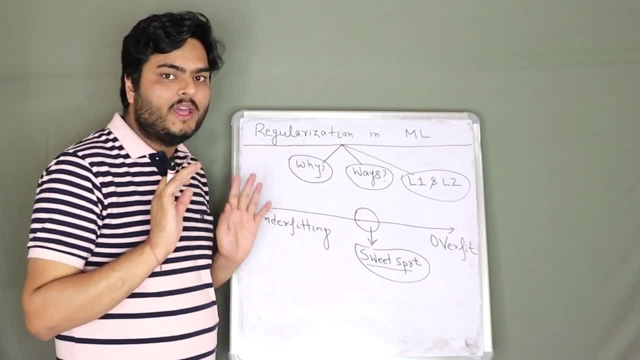 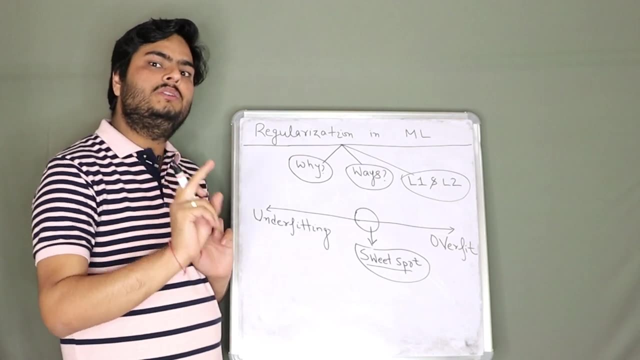 a balance between these two. okay, and that balance point is: i have written here the sweet spot. for all the data, this sweet spot might vary. now, i had created a video on bias variance trade-off and that is what i explained just now. these kind of models have high bias. these kind of models have 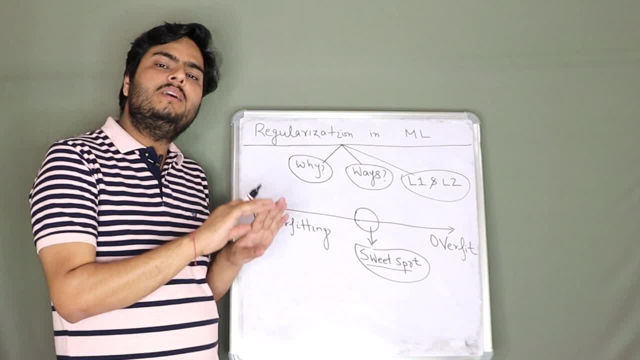 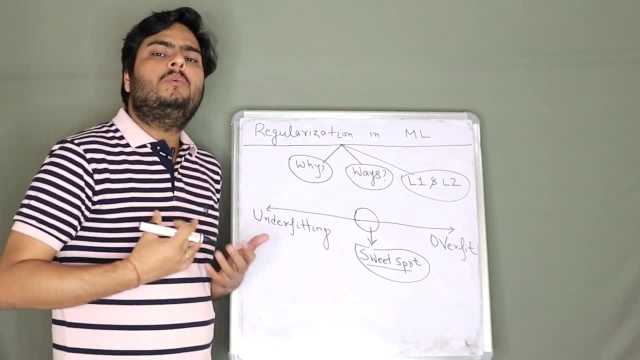 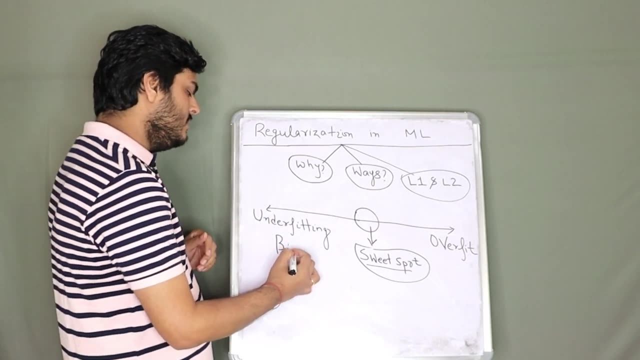 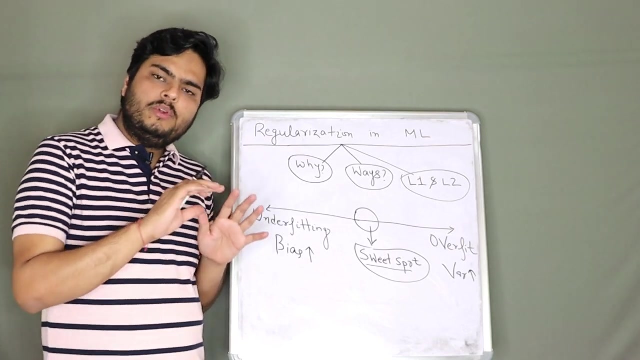 high variance and what we try to balance: bias and variance. you can see the link here. you can watch the detailed video as well. now, what type of model will have high bias and what type of model will have high variance? so let me write: here bias is high and here variance of the model is high. so if we talk of 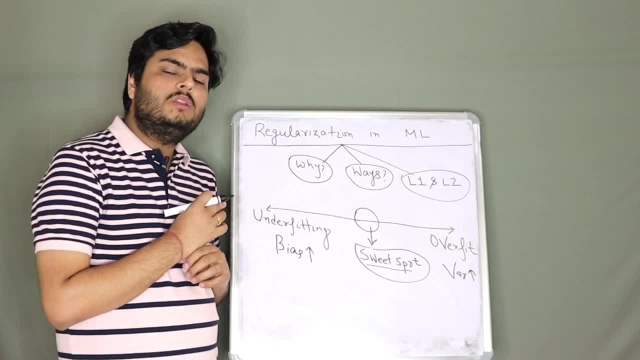 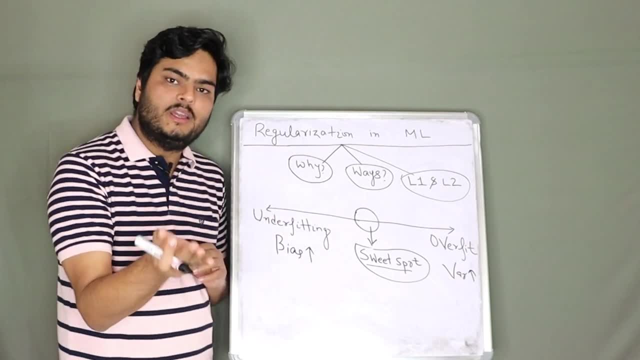 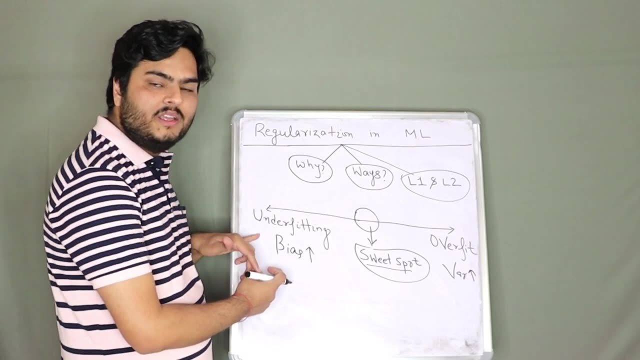 regression based models. right in regression based models, model assumes the form of the data. it assumes there is a linear relation between independent and target. so there is a bias. there is a parametric model. hence these kind of models have high bias. you typically see, the model has high bias and it assumes that there is a linear relation between independent. 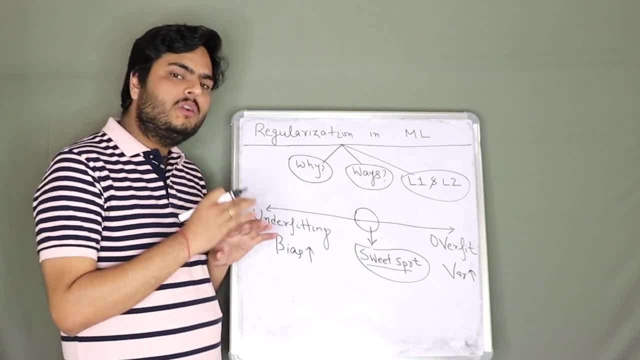 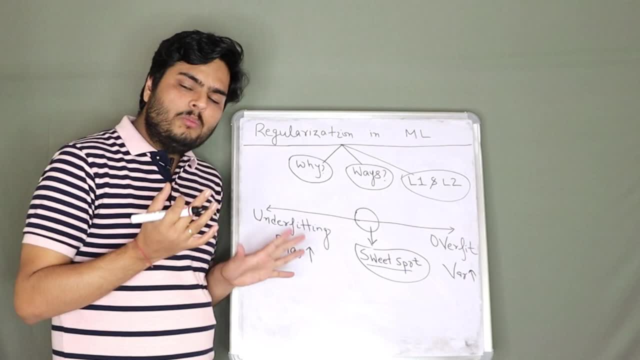 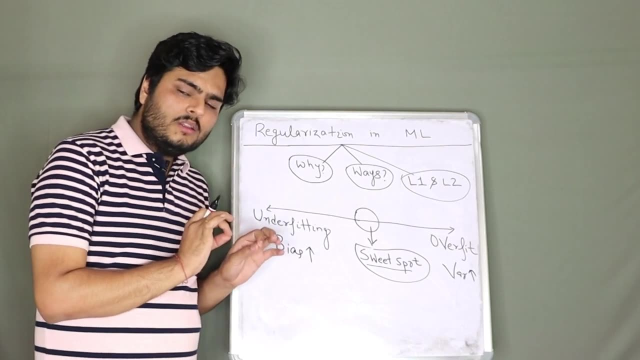 and target. so you can see that regression models will not give you very good accuracy on trend data, also on new test data also. okay, what kind of models will have high variance? the model which is free to do whatever it want to do. understand, guys, this very clearly. there are few models which is free. 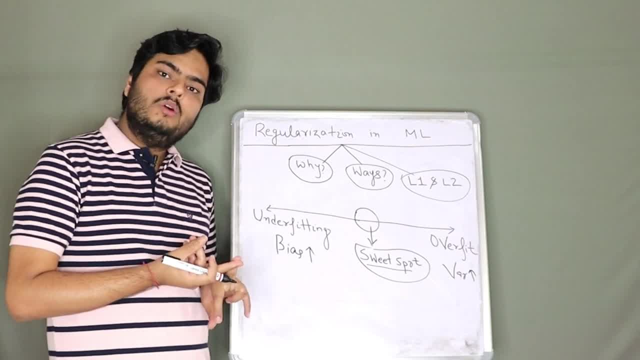 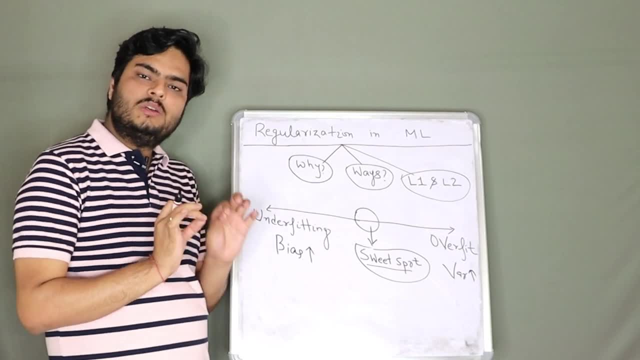 to do whatever it wants to do, for example, decision trees, for example your plain neural networks, all these models and until or unless you don't do some regularization, some parameter tuning, some pruning, all these model and a free model. they don't assume any form of the data. 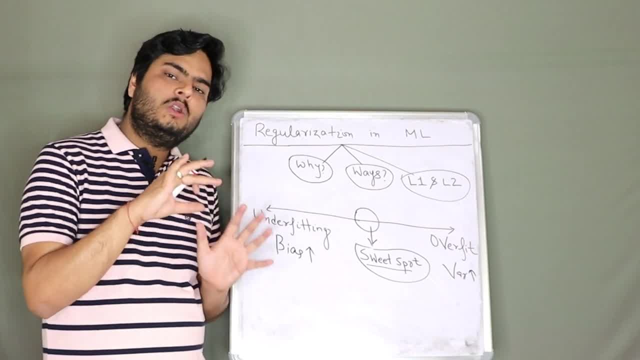 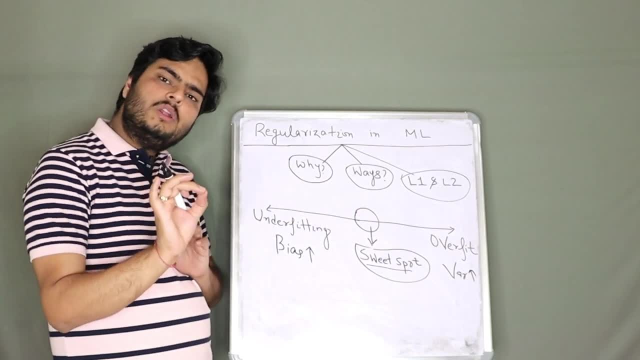 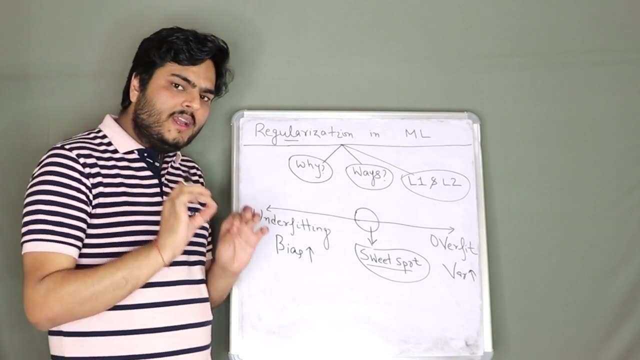 these kind of model. typically, if you don't control the parameters, typically it will tend to give high variance. okay, now let's talk about few models in particular and try to understand how do we regularize that model? to rewrite rate again, to find this sweet spot. we need to regularize the 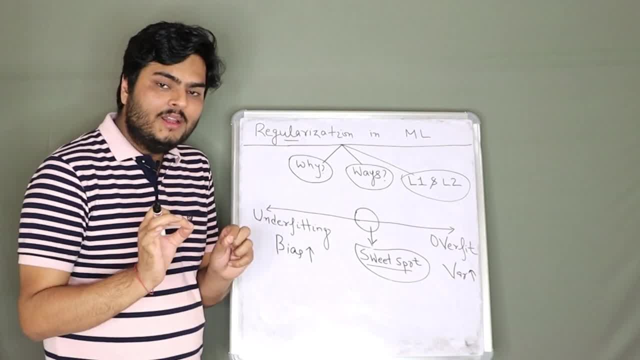 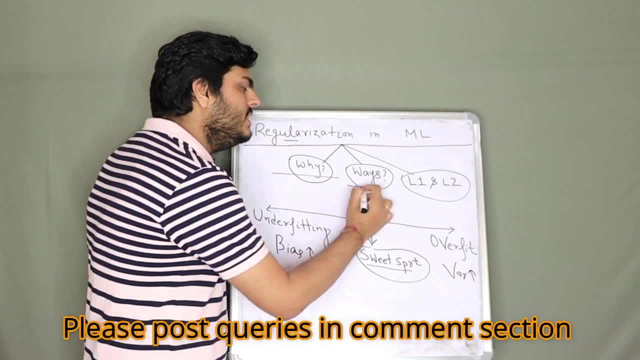 model. okay, to regularize the model, we need two sweet spots. okay, so the third is recessive. so to the model. there are different ways. okay, the why part we discussed. next question comes: what are the different ways in which regularize? we always hear about l1, l2. are there other ways? so, guys, l1. 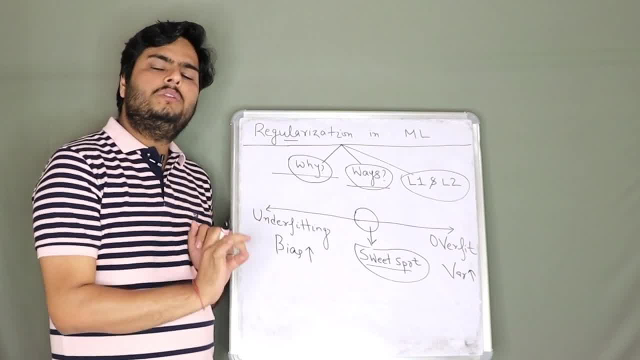 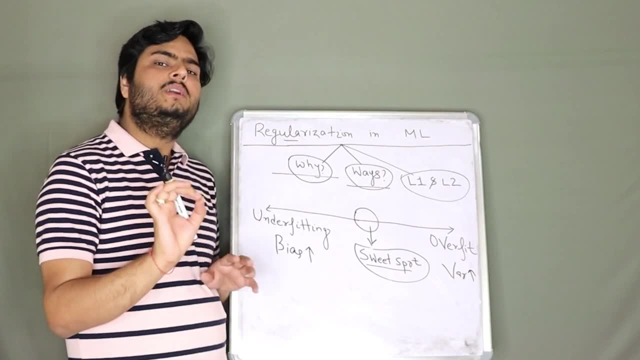 l2 is applicable to regression models only. if you talk of decision tree models, right then you would have heard of bagging and boosting techniques. those are nothing but regularization techniques. okay, what we try to do when we fit a random forest, what we try to do when we put a ada boost, 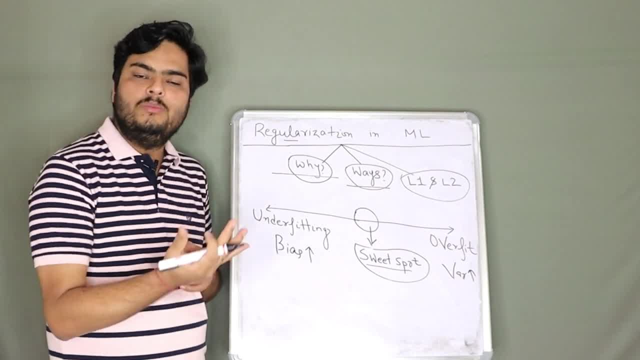 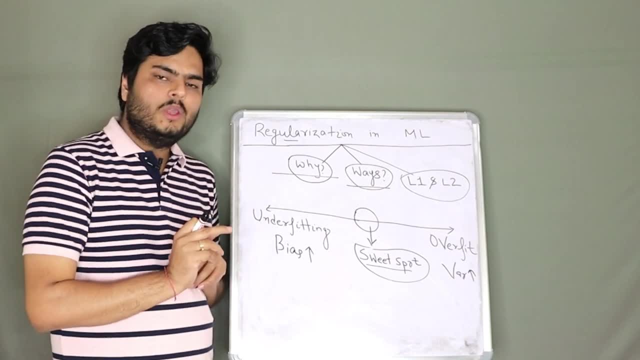 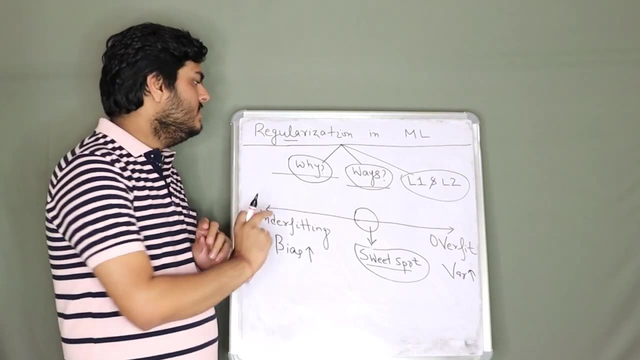 we try to reduce the variance of plain decision tree model, right? if you go to deep learning models, right, you would have heard of something known as dropout layer. what is the use of dropout layer, guys? dropout layer is nothing but a method to regularize the deep learning model, or a method. 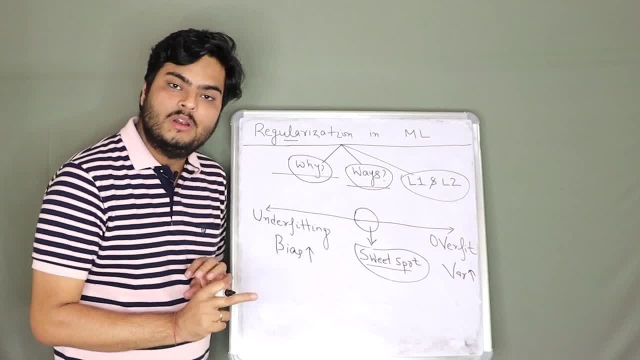 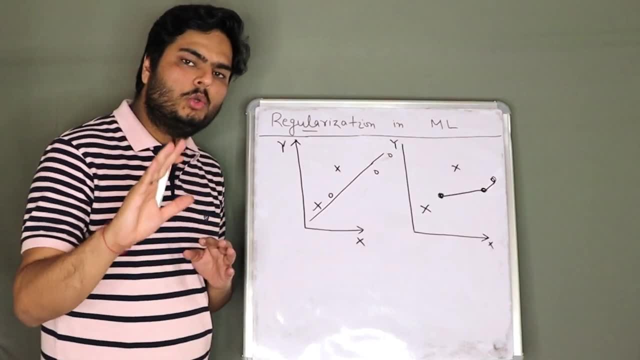 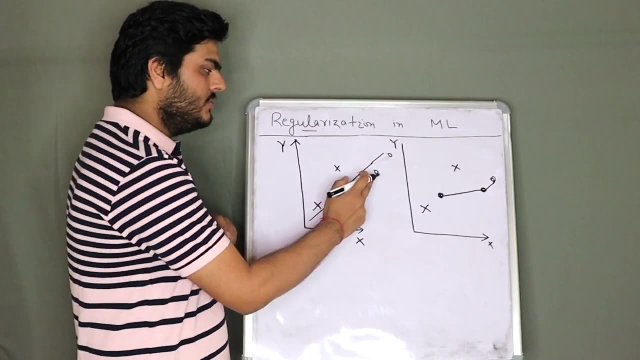 to prevent overfitting of the deep learning model. you. now we will go a little detail about l1 and l2 technique. okay, so, guys, here i have drawn two images. okay, left hand side chart is about your underfitting of a model. so all these dots are. 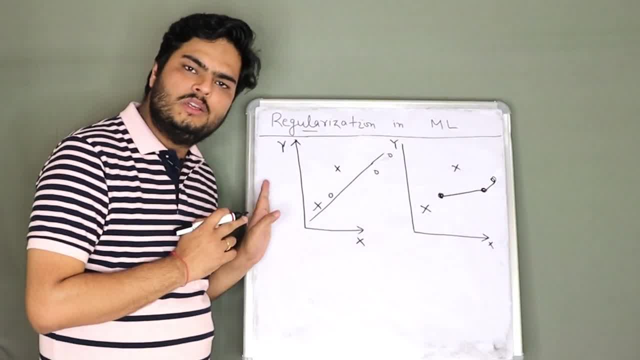 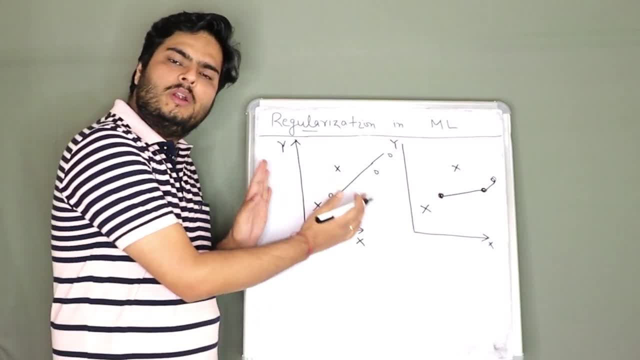 your training data and cross is your test data. suppose we are fitting a linear regression model. okay, cross is your test data, all the dots are your train data, cross is your test data. so what is happening in this one is model is kind of not fitting properly to the data. just see the 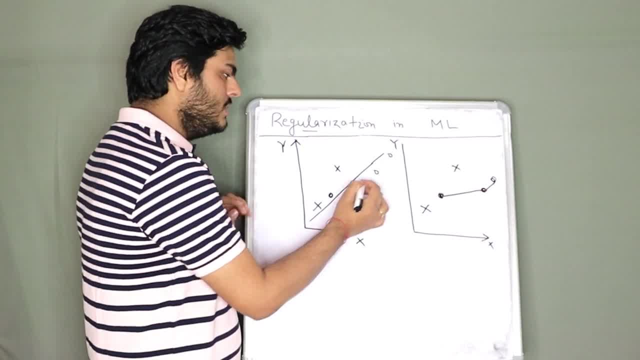 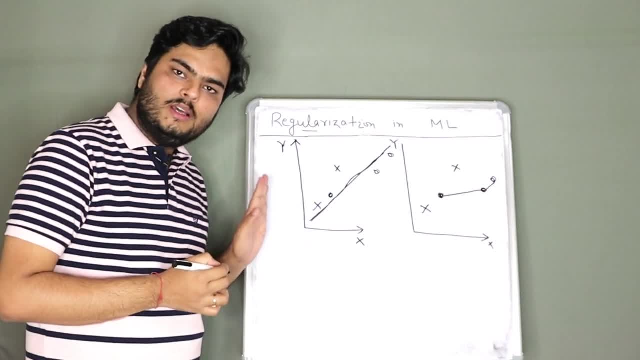 dots are not fitting properly to the data. just see, the dots are not fitting properly to the data now because dots is the training data. okay, so one dot, two dot, three dot. so model is this? one simple line like this. okay, this model may not be fitting on the train data, as good as this is fitting if you. 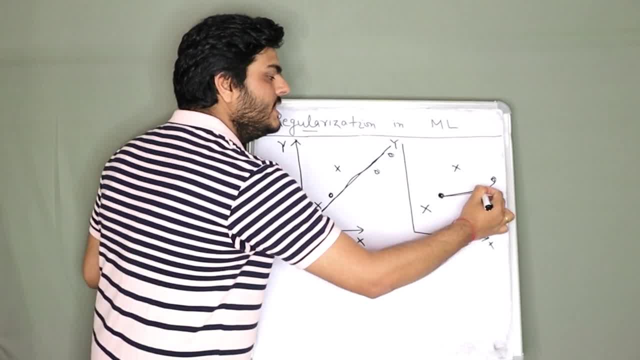 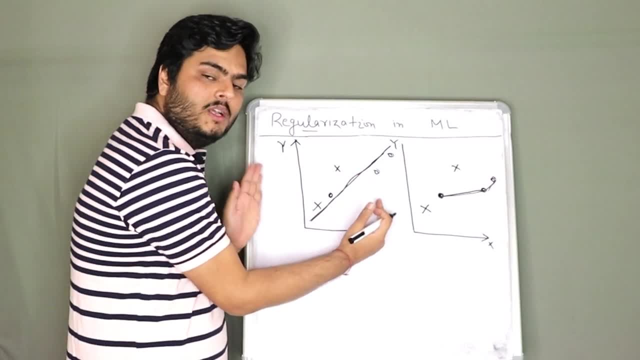 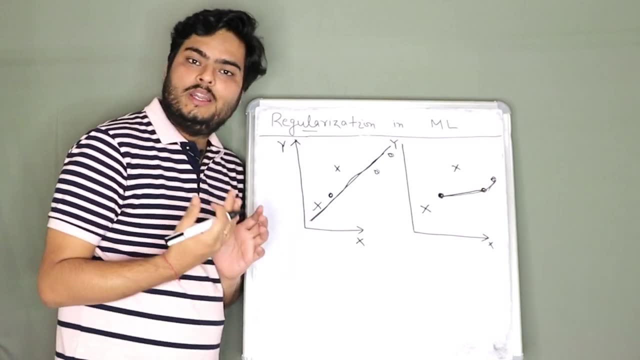 see one, two, three dots right. so it is going like this kind of hugging the train data, kind of remembering the train data. the problem with this model is it will not give very good training accuracy and test accuracy. also, probably it is not fitting to the data very well. the problem with 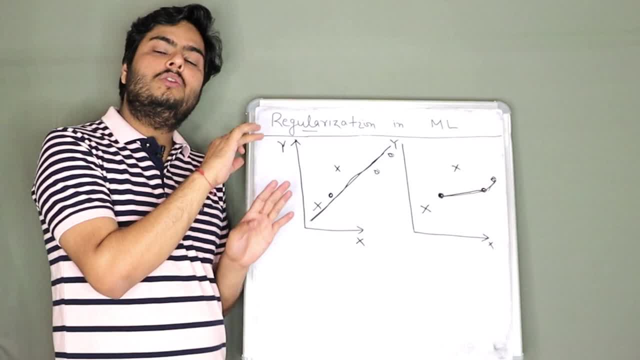 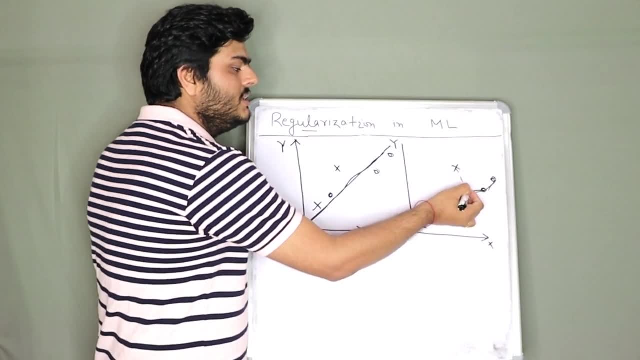 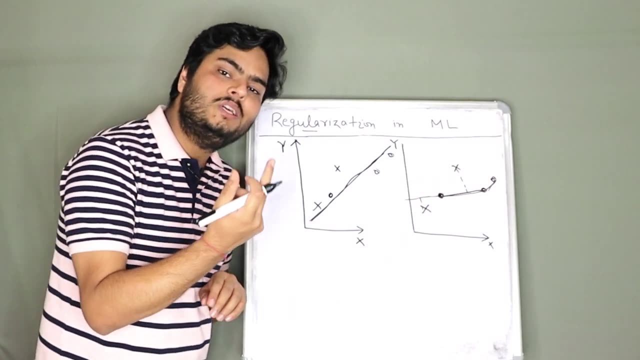 this model is. though it is fitting to the training, it is not going to do any good on the test data. so suppose i want to predict on this data. if you see these distances will be too high, okay, these distances will be high, which means model's accuracy will be low on the test data. 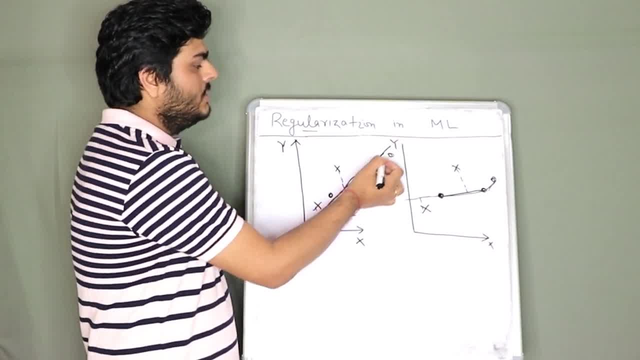 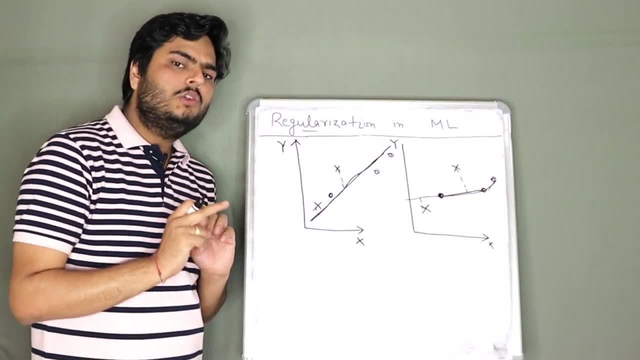 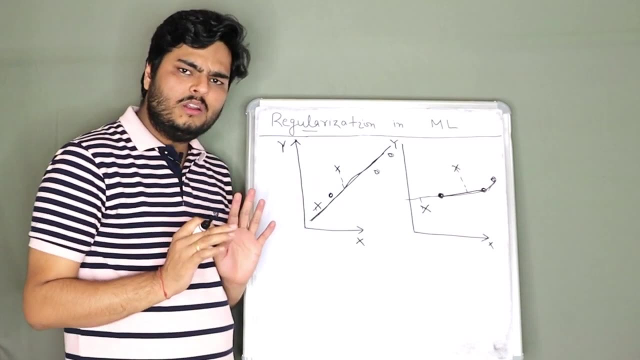 on the other hand, these distances will be low, which means model accuracy will be very low and accuracy will not be that that bad. so this is underfitting. this is overfitting. what we try to do here in regularization is we try to find a midway. i was showing, using, showing you the sweet spot. 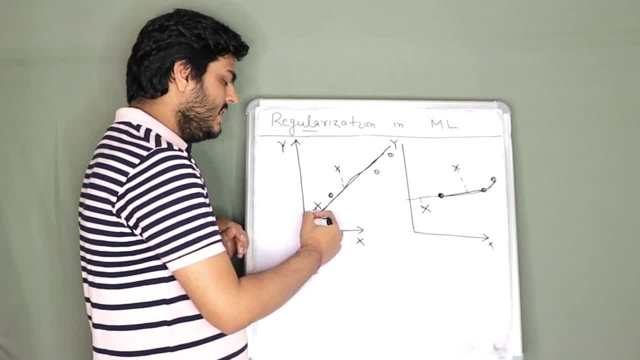 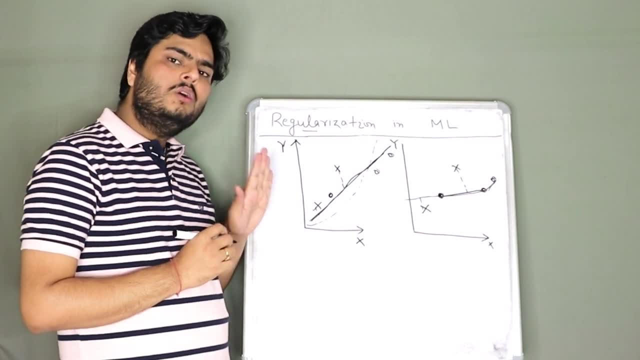 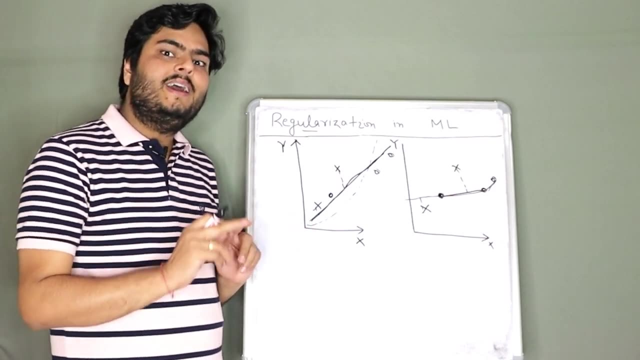 right. can i have a curve, something like this, which is not very complex and it does the job? can i have a curve like this for that, since this is a regression based model, so it's all about mathematical equations and it's all about coefficients. now imagine if it's a tree based model. we don't talk. 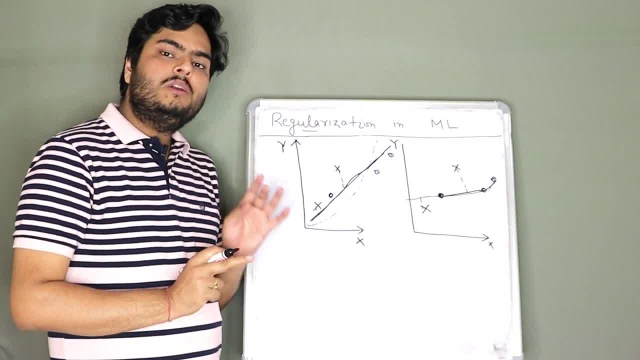 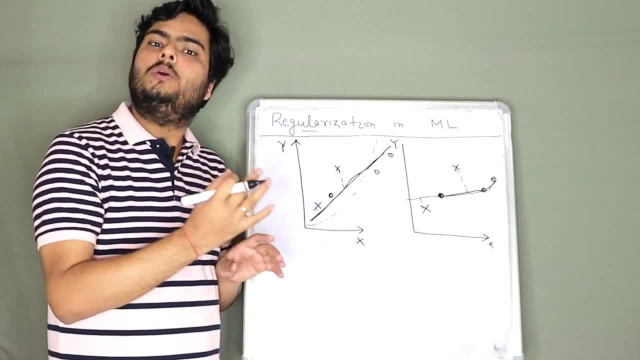 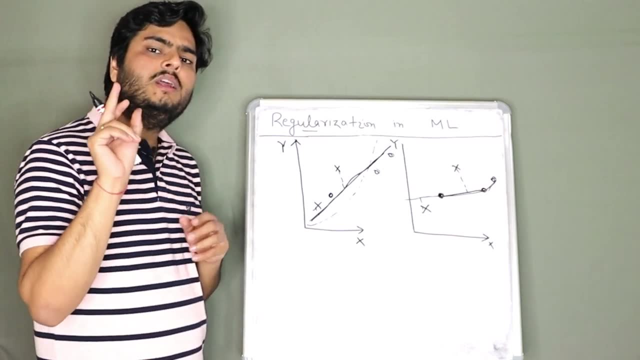 about coefficients. i already explained. we talk about bagging, boosting and sampling those kind of things. if it's a layers in deep learning model, we talk about layers like dropout layer. here it's all about coefficients. so we control coefficients. so how do we do that? there are two ways to do that. 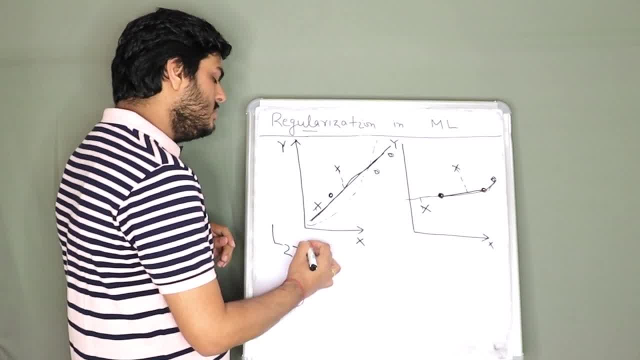 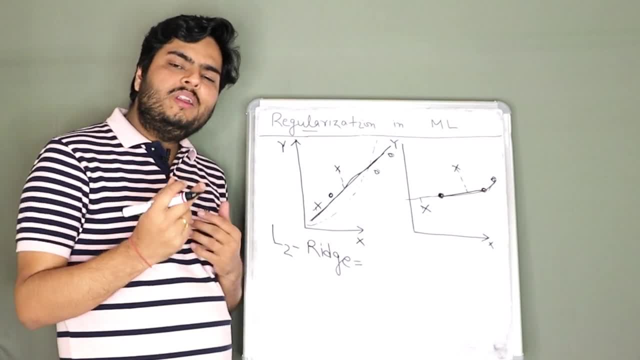 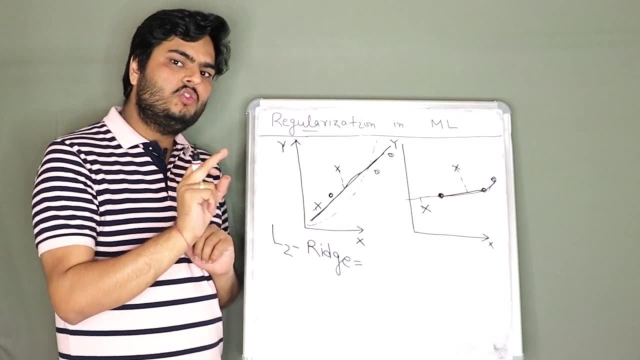 one is known as l2 regularization and also known as regression, r, i, d, g, e. okay, here what we do is we redefine the loss function now, loss function and cost function. i have explained in detail. the link is here, guys, you can watch to keep it high level. 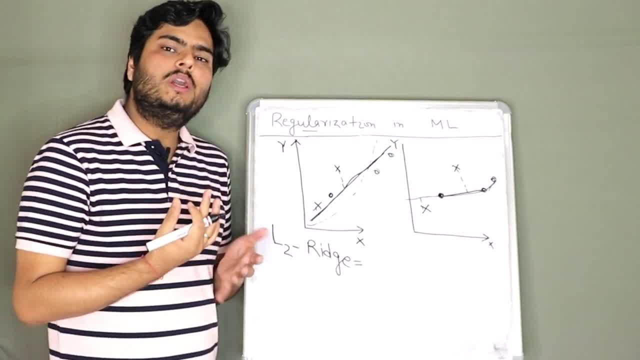 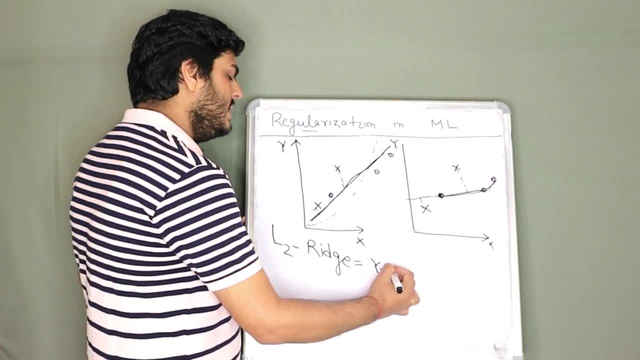 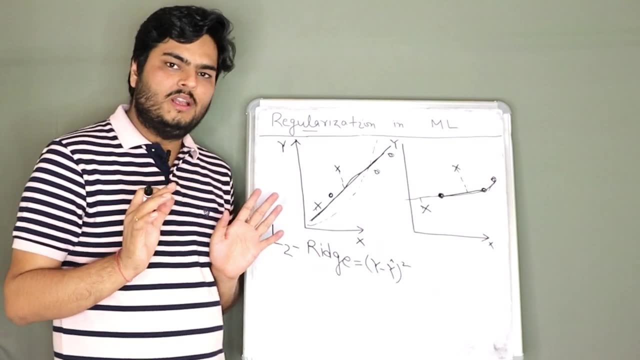 loss function is nothing but the function which is optimized to gain the coefficients values. what is that function typically? typically, that function is y minus y hat. y is actual value, y, hat is predicted value. whole square, residual sum of squares, nothing else. okay, this function will be tried to minimize. 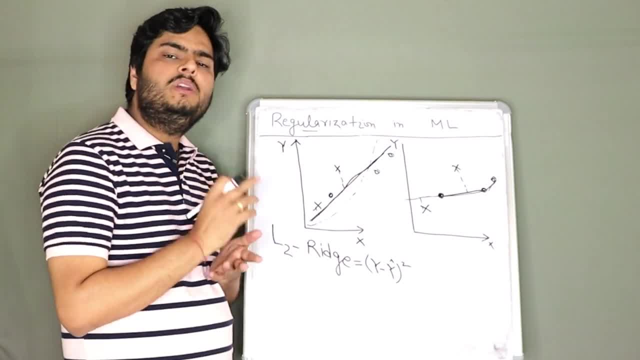 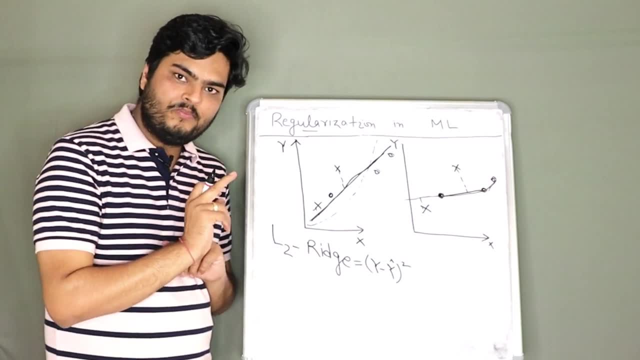 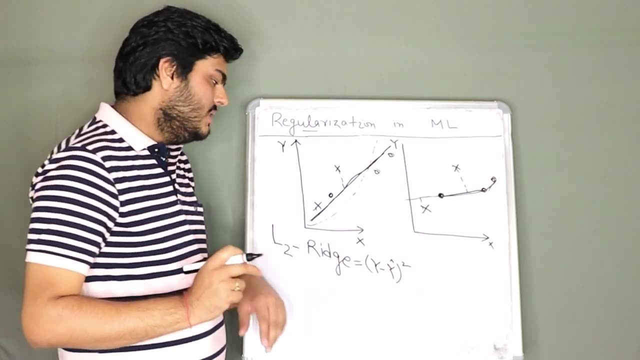 where from y hat will come. y hat is nothing but beta 0 plus beta 1 x. 1. correct, where beta 1 is your coefficient, beta 1 is your slope right. so in l2 ridge regression, this cost function, i am writing the cost function here. the cost function will have an additional term. that term is known. 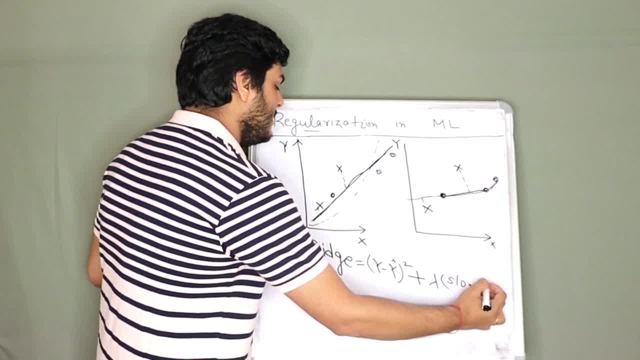 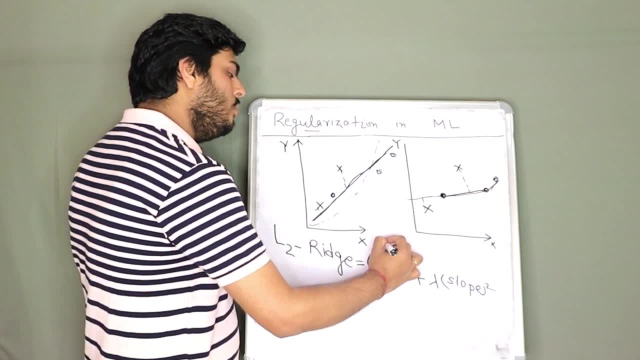 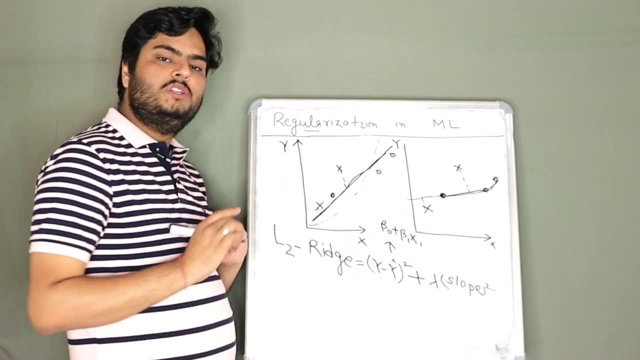 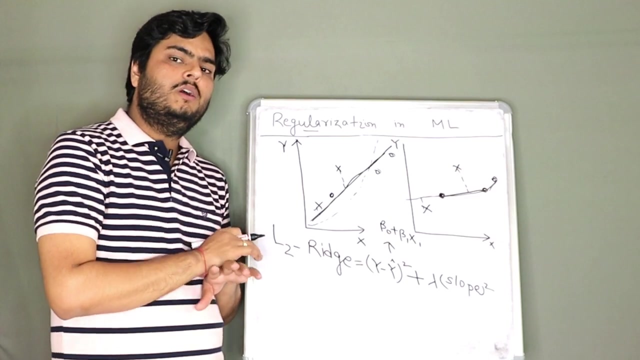 as lambda into slope square. what is this slope? this slope is nothing but the coefficients. so if you think this y hat has beta 0 plus beta 1 x 1 for first observation, then this slope will be this beta 1.. what will happen due to this, guys? what will happen due to this? what happens if this line? is very steep. Jakos surely will get going and do it way steep in this point. so if you think that leadership is very deep, if you think that lambda x is lambda, what will happen if lambda x is actually 현caikt and so on will not be a real slope負 Int application is that. 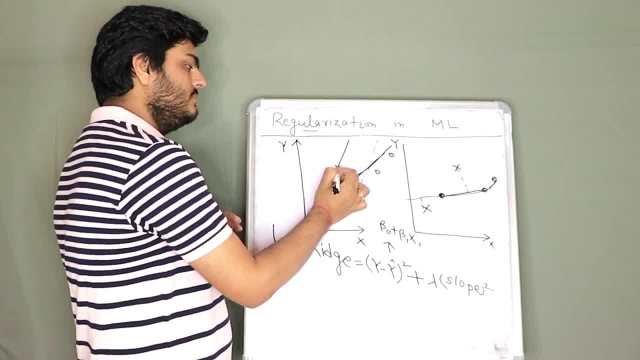 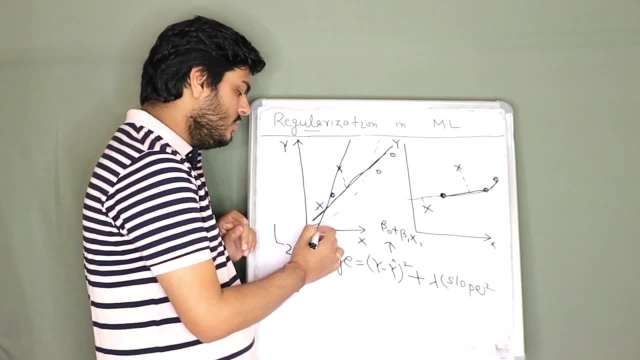 more moment before lets talk a little bit. the vector here again. Very steep means like this. What will happen in this case? In this case for a small change in x, also y will increase by a bigger margin if it's a steep curve. 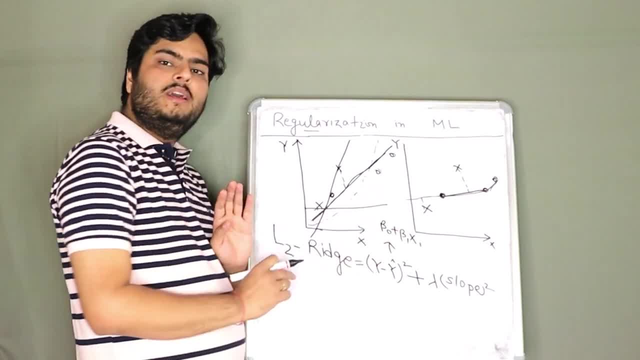 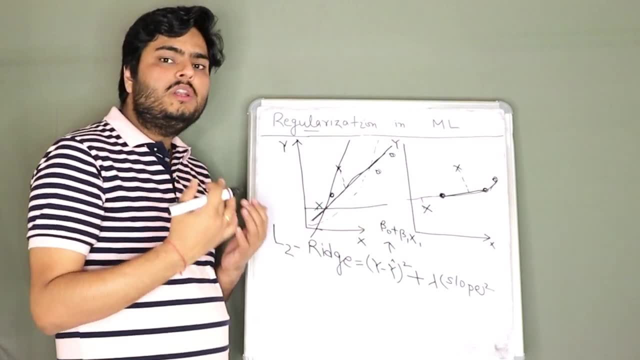 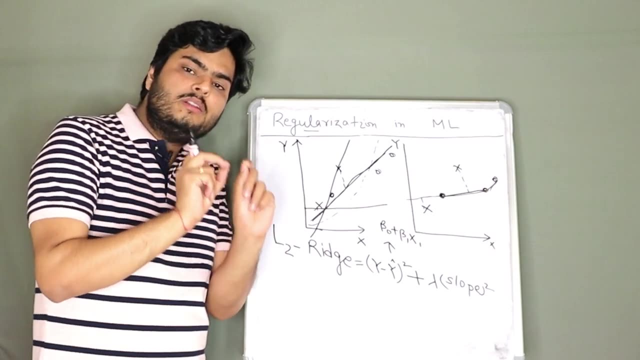 If it's a flatter curve for a small unit, shift in x, y will not shift by that much. So it's all game of these coefficients. Now it depends on us how much this value of coefficient we want, And that is what we regularize to find that sweet spot. 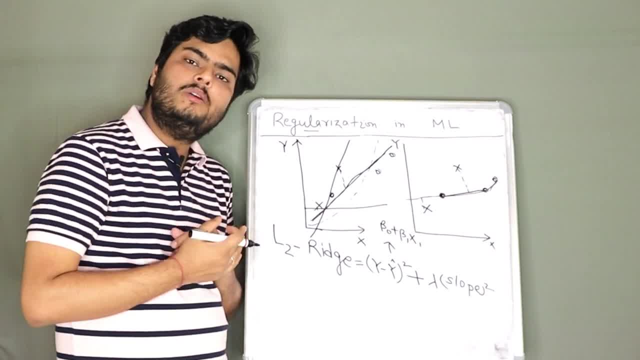 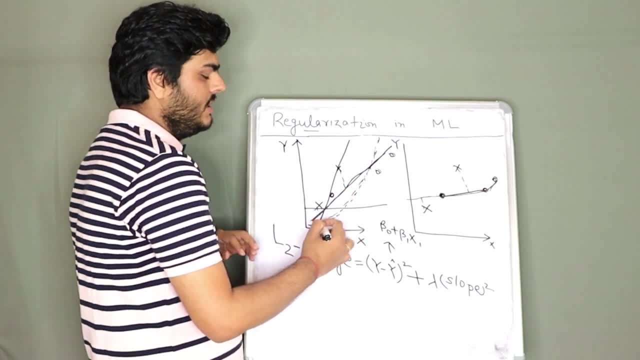 This coefficient will only make your model underfit or overfit. I was talking about this dotted curve. We want to have this dotted curve kind of thing which will give me a sweet spot. How you will have that sweet spot? You need to have the right coefficient. 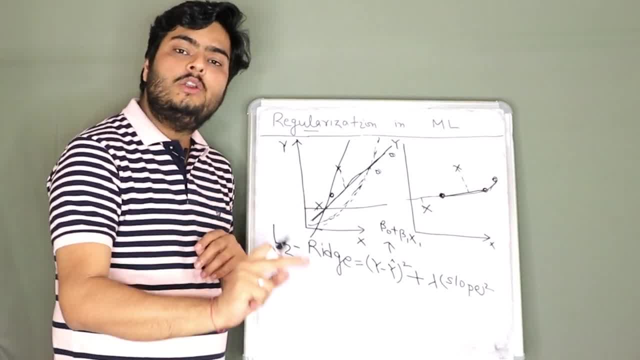 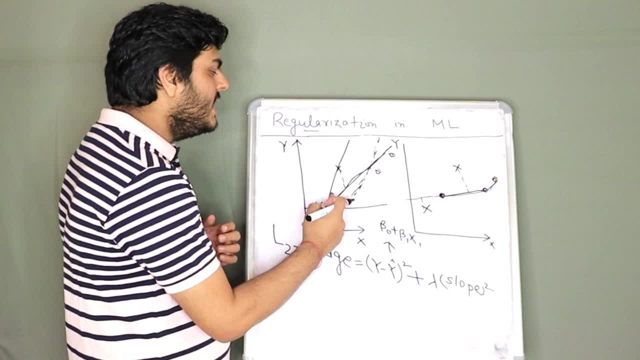 What is the right coefficient? The coefficient which is not too high and not too low, based on your data? How do we know What is high and what is low for my data? I know by looking how y is responding to different x's. 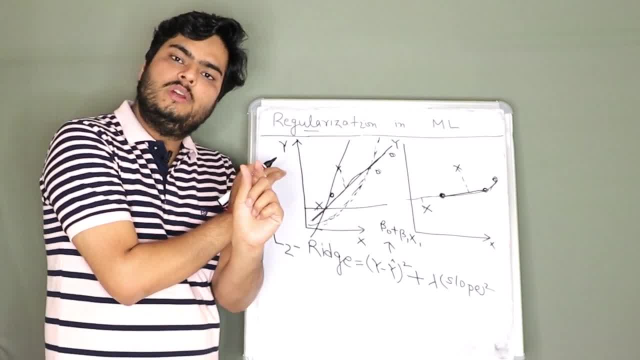 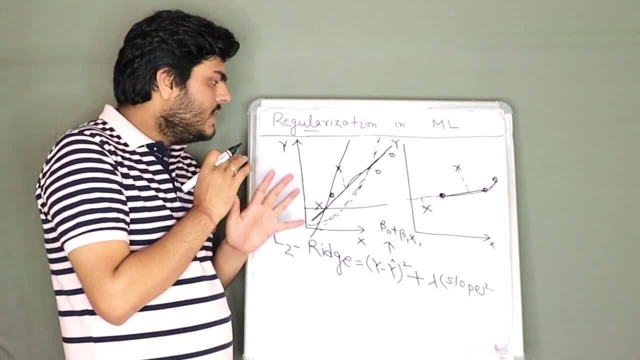 So, as I told, this is a steep curve: More shift in y with small shift in x. This is a flat curve: Less shift in y with less shift in x. So what will happen when we use this L2 ridge regression is: 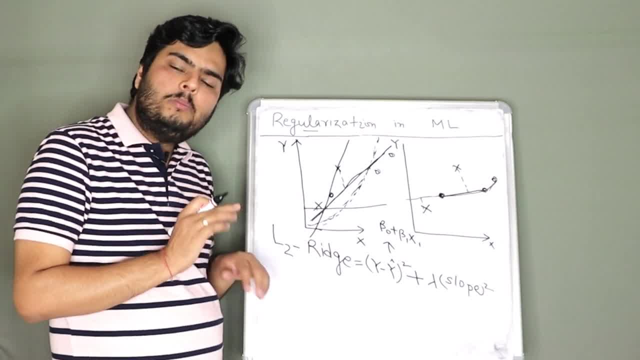 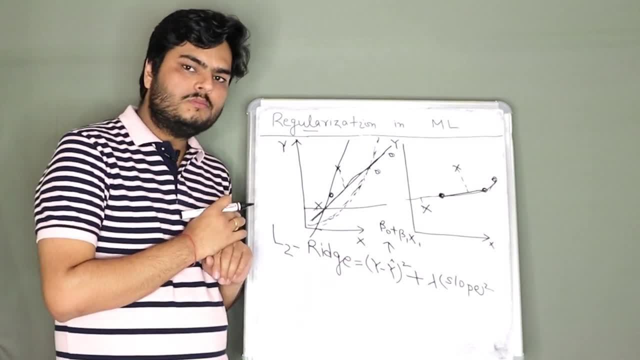 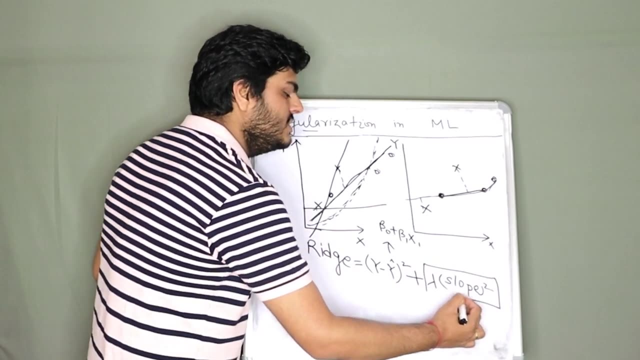 the optimal value of your loss function will be derived based on proper coefficient value. So what will happen is, if your coefficient goes beyond the limit, then this term will shoot up. See this term, guys. If your slope is high, then this term will go up. 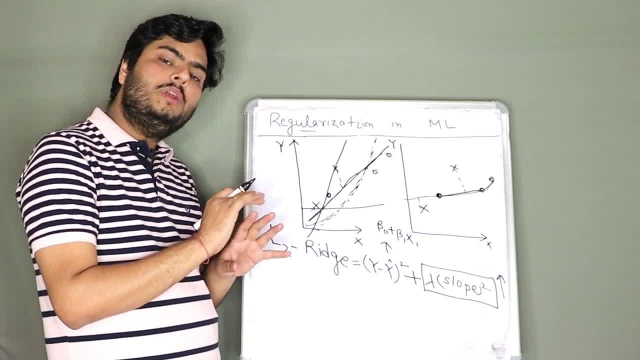 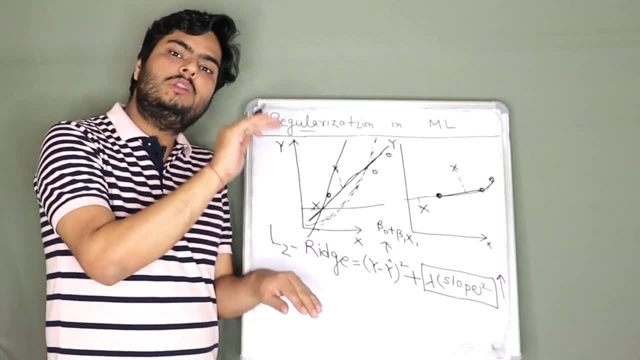 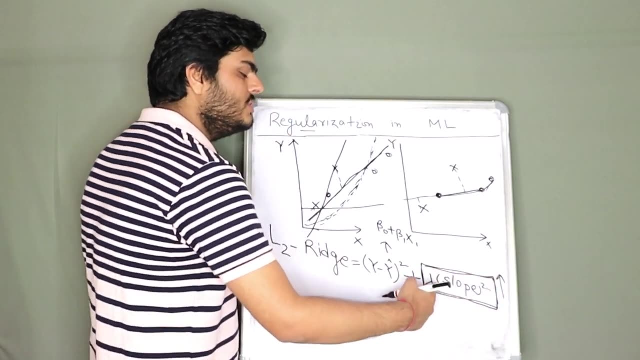 If this term goes up, then your cost function value will go up, which is not what model wants to do. Model wants to keep the cost low or the loss low, So this term has to be low. This term cannot be high and lambda is a fixed number, guys. 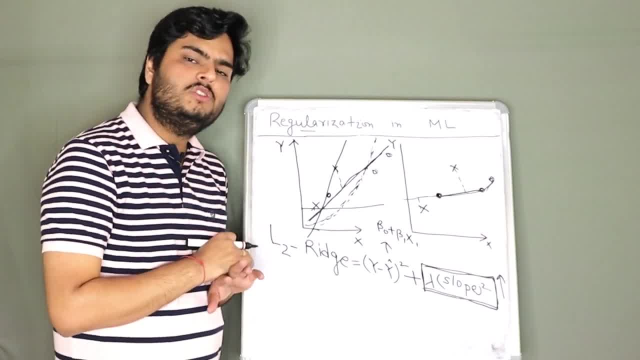 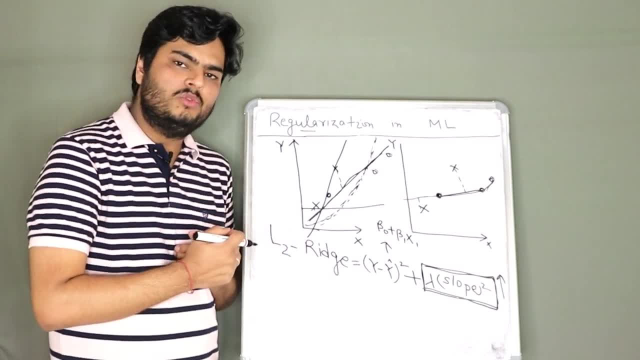 You can pass in the SQL and when you call this model, let's start with 0.01 or something like that. So lambda, you can pass it like lambda is a parameter You can tune like you tune in gradient boost and all. 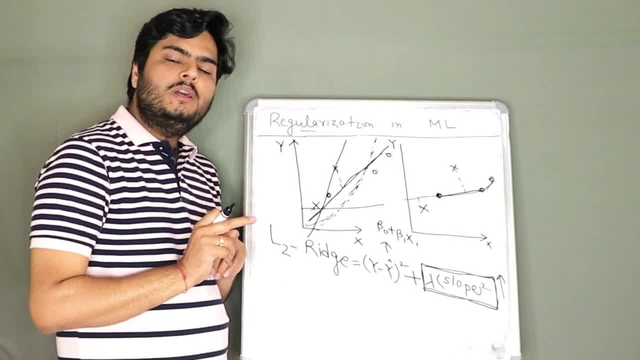 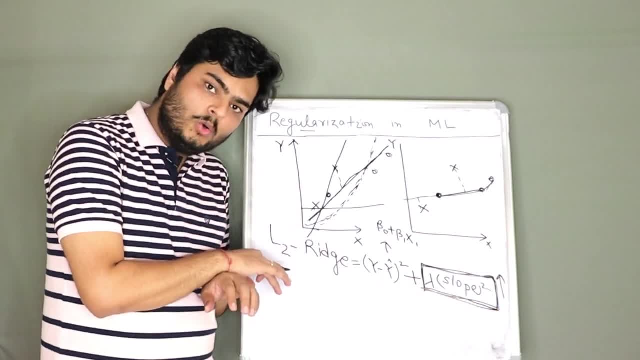 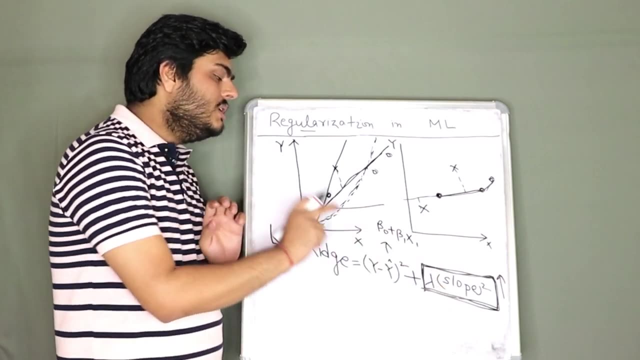 Okay, but this slope is the important thing here. This entire term has to be low. Then only your cost function value will be low. and to keep this entire function as low, entire thing, entire This, whatever is in this box, to keep this term as low, 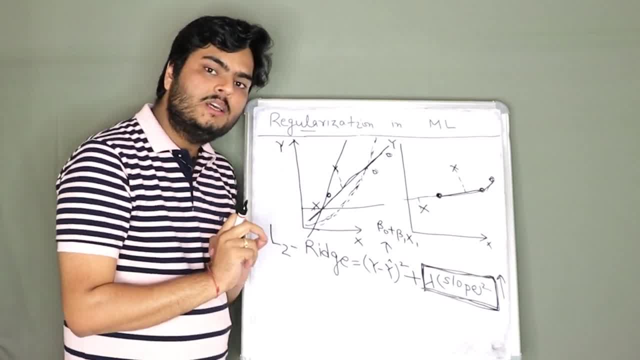 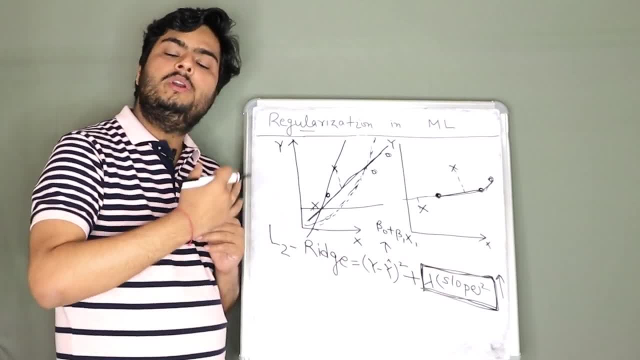 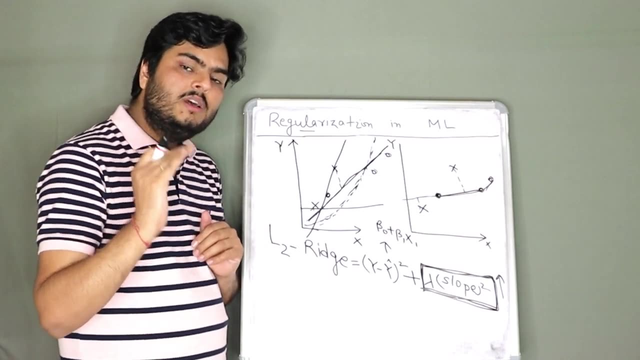 Your coefficient should be tuned in such a way that you know this entire thing. value becomes low. for that to happen, Your coefficient cannot go beyond the limit. Understand this, guys. your coefficient will not go beyond the limit because if it goes, the value of loss will start shooting up. 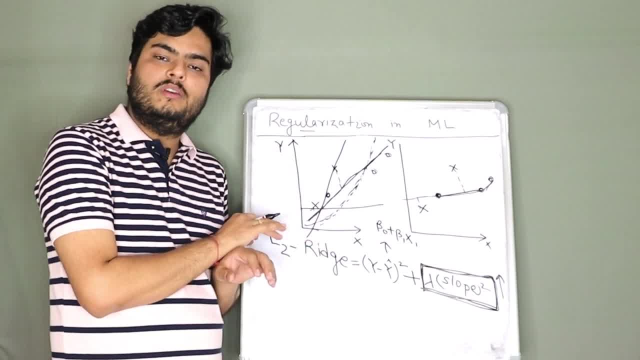 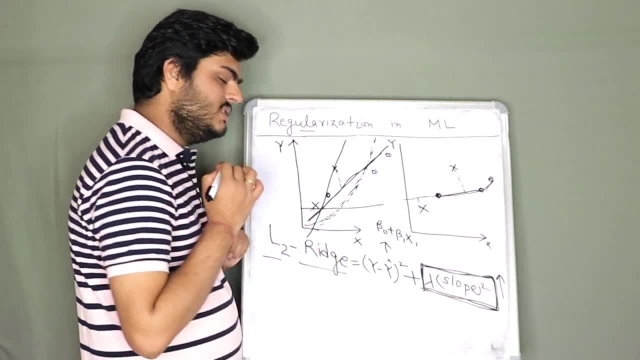 Hence we call this method as shrinkage- coefficient shrinkage. It will not allow your coefficient to go beyond the limit, and that is what L2 regression, or ridge regression, does. This is a regularization of your coefficients. Why were we are regularizing coefficients. 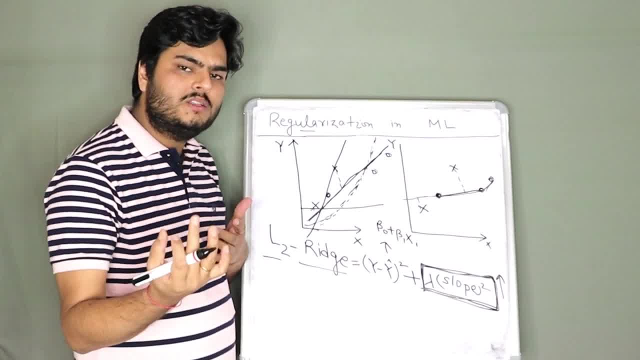 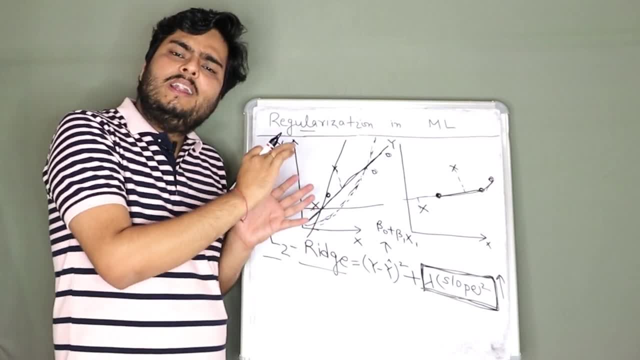 Because it's a regression model. If it's a neural network model, we will do something else. It's a regression model, Hence coefficient regularization right. How to regularize the coefficient: Add an additional term in the loss function lambda of coefficient square. 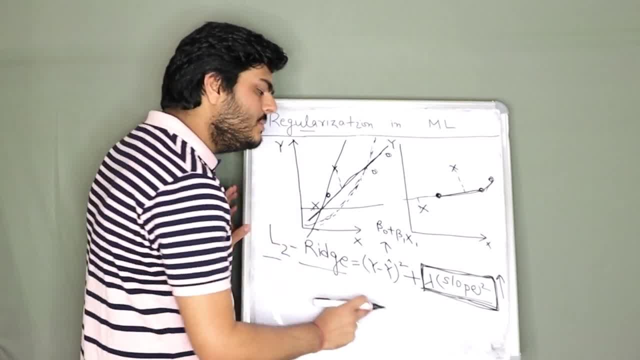 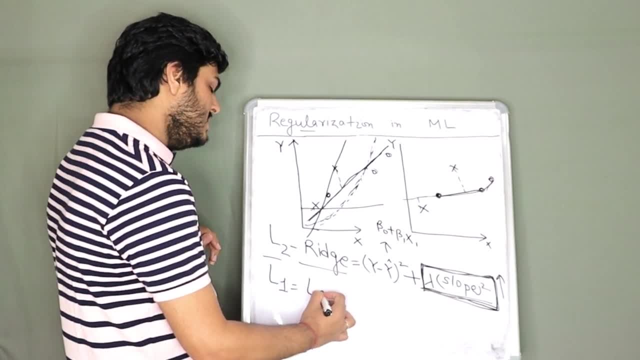 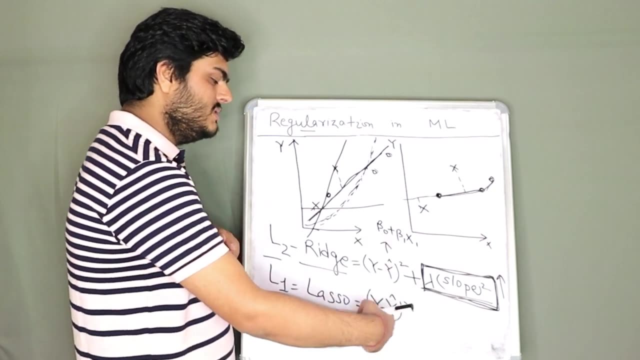 and it will be automatically taken care. Okay, this is about your loss function of ridge regression And one minor difference if you compare with lasso regression is your cost. function remains same. This will obviously repeat for all the observations. guys, I hope you are getting it plus lambda into modulus of slope. 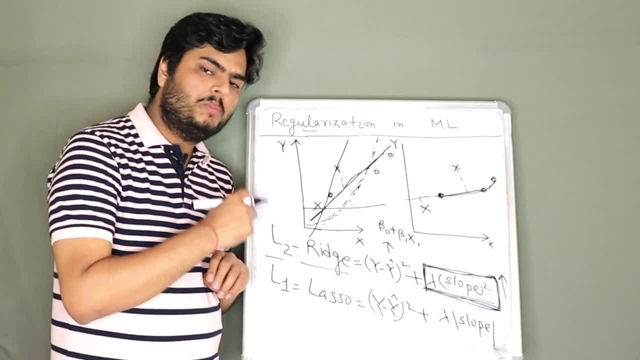 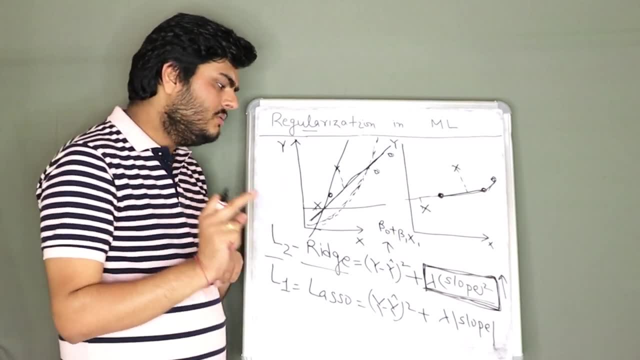 Modulus of slope means some slope can be positive, Some slope can be negative, Some beta values can be positive, Some beta values can be negative. So so that it does not cancel Out each other, We take a modulus. If there are more betas, we add here. 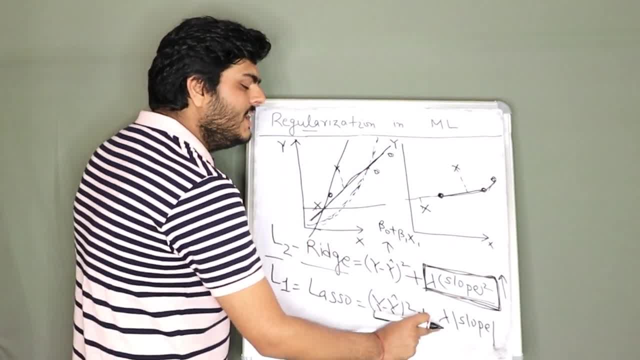 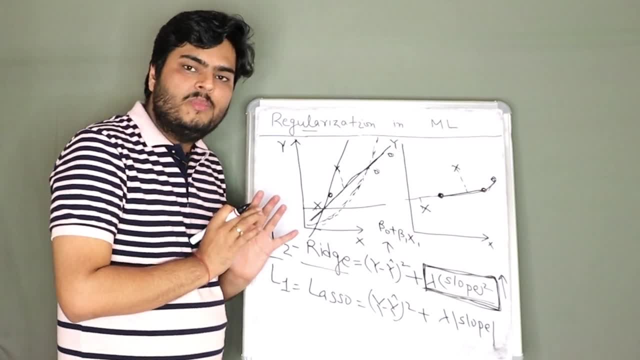 Okay, beta 1 plus beta 2 plus beta 3. multiply that by lambda. Lambda is again a hyper parameter that we need to tune based on our data. The purpose remains the same here. Also, we are shrinking the coefficients. We are shrinking the coefficients. 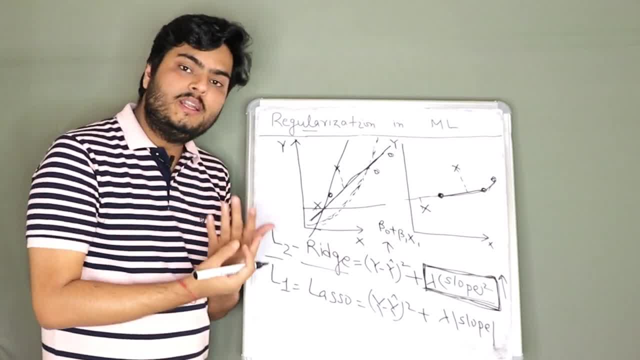 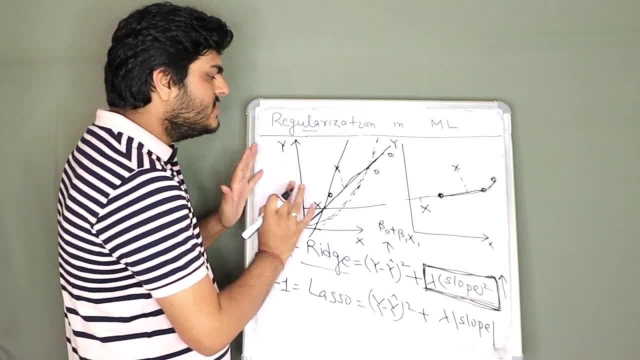 Okay, by how much? that depends on how our data is, where our optimal lambda is and where our optimal value of the data is, The coefficient is. but the purpose of this entire exercise is to regularize the model So that we find that sweet spot. 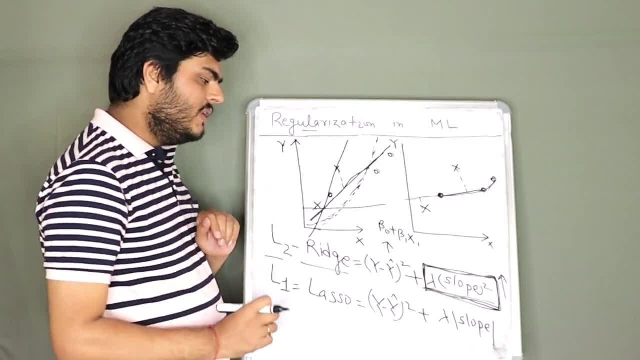 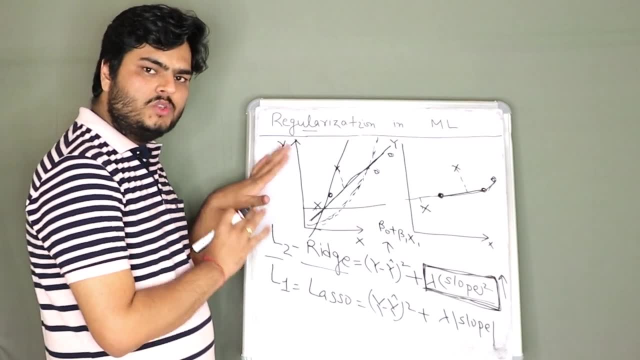 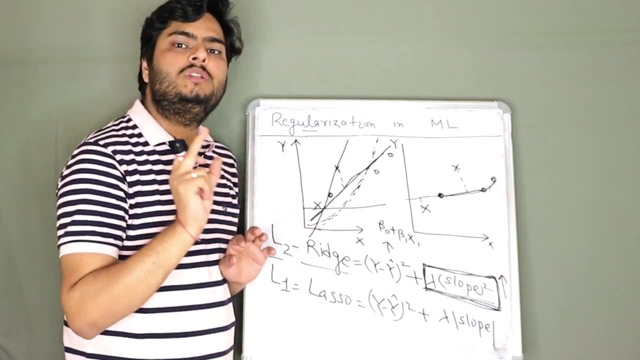 Okay, and there are slight differences between l1 and l2 regularization, which I am going to cover in next video, because this is getting little longer Now. I will just summarize what all we discussed so that it remains in your mind. regularization: a process to find the optimal point in the model. optimal point means sweet spot, bias, variance, balance. 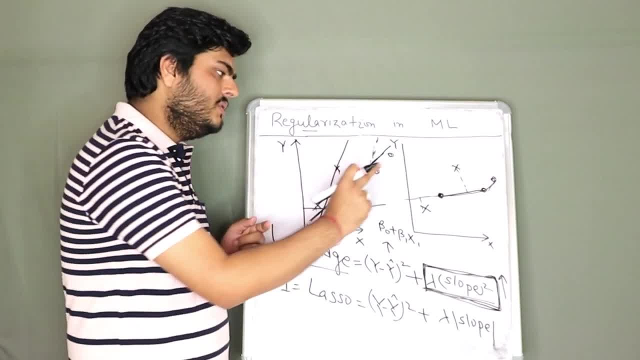 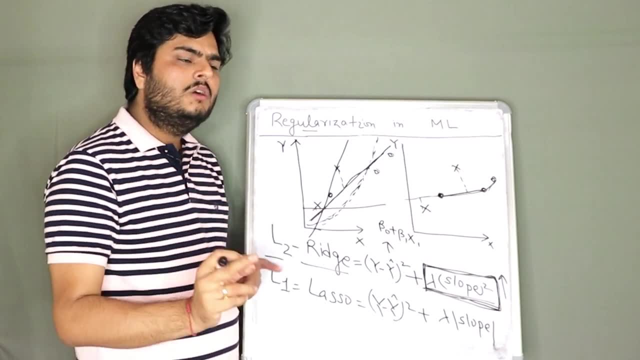 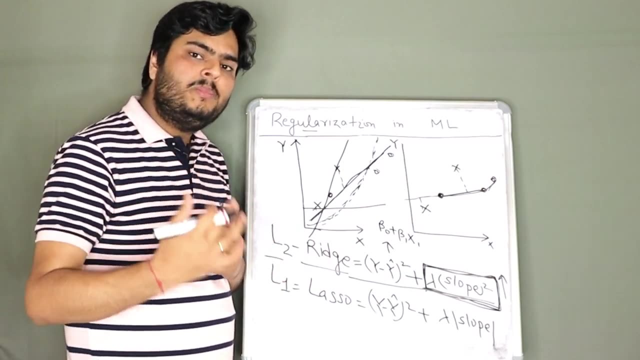 Different types depend on the model. If it's a regression, l1- l2, if it's a decision, tree, bagging, boosting, stacking, if it is a neural network dropout and these things- l1- l2 regularization. What we do, we tune the cost function of simple linear regression and we add another penalty term. 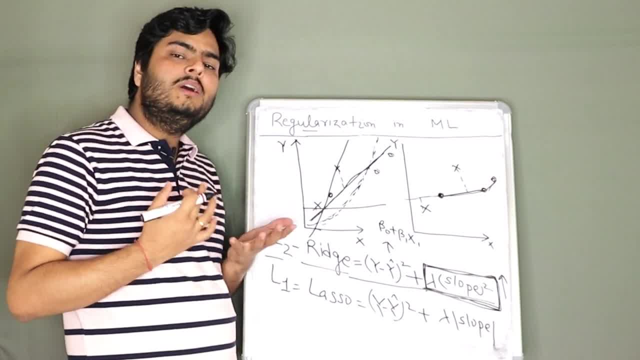 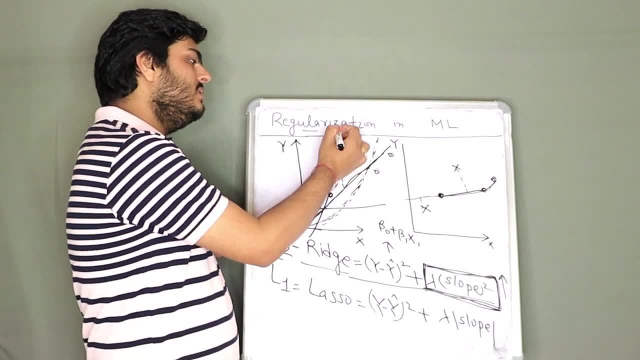 Why we add this term. We add this term because we want to have a shrinkage. We have. we do not want the coefficient to go beyond the limit so that it is difficult to control. We do not want a very Deep curve. Okay, one more thing.